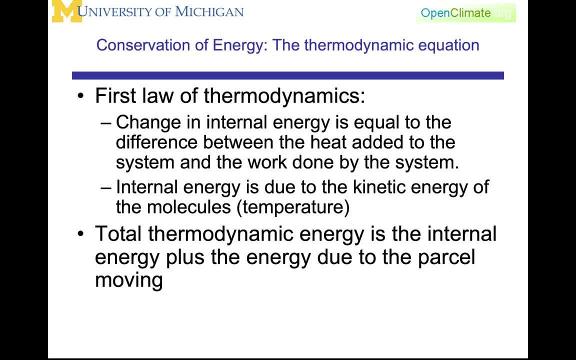 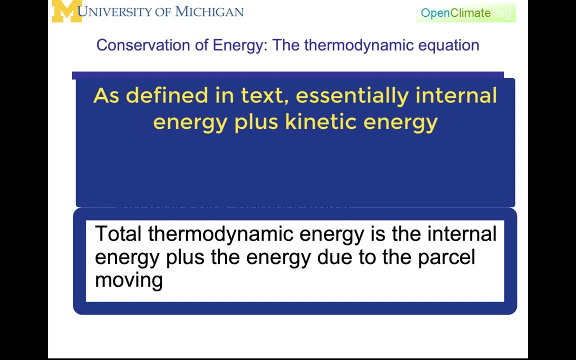 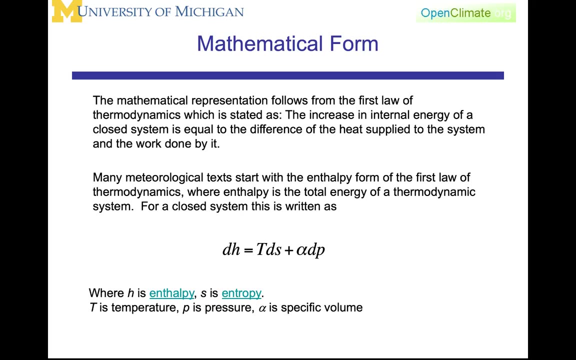 and since heat and work are both energy, you can see the natural relationship to internal energy. Total thermodynamic energy is the internal energy plus the energy due to the parcel of air or to some other piece of matter that is moving Mathematical form of the thermodynamic energy. I will write like: 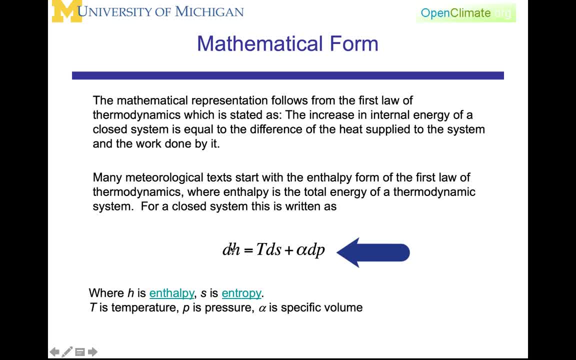 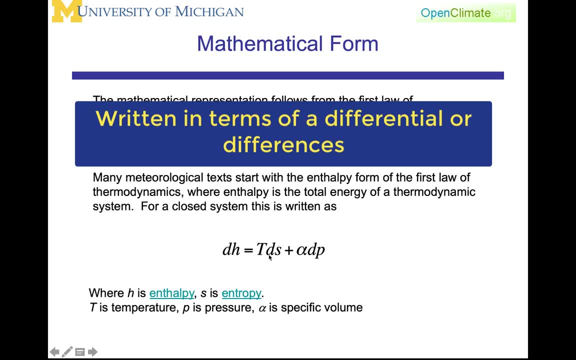 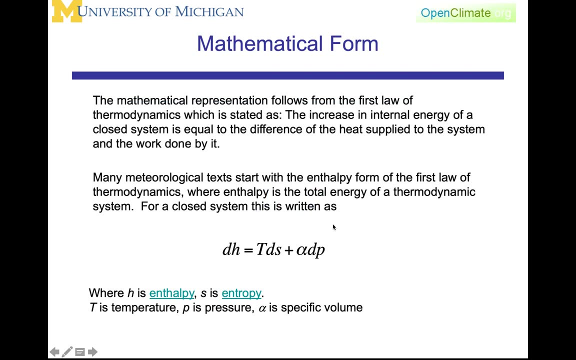 this where we are writing. in terms of a difference, dH is equal to another difference with dS times, alpha, dp. Now I will go through and define these. So the mathematical representation follows from the first law and says that the increase in internal energy of a closed 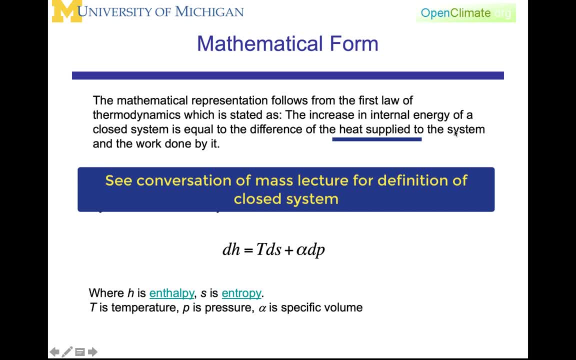 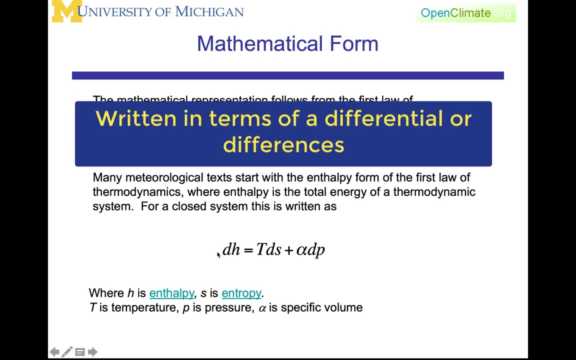 system is equal to the difference of the heat supplied and the work done. And since we are talking about the increase or the decrease or the change in internal energy is why we write this in terms of these differentials, where here the d is, as in calculus, dH, And. 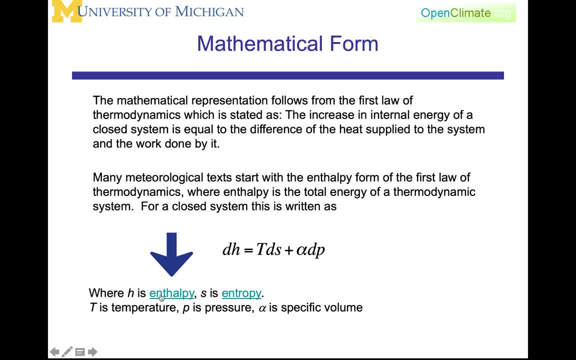 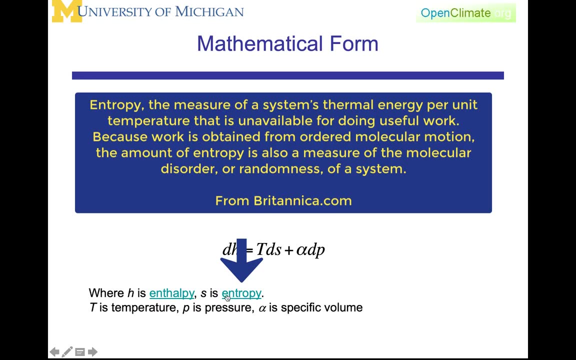 what H is here is enthalpy, And enthalpy is essentially a measure or a type of heat, And it's equal to the temperature times dS times- alpha dp And the temperature times dS times- alpha dp, And in this case S is the entropy, And entropy is often said to be a measure of. 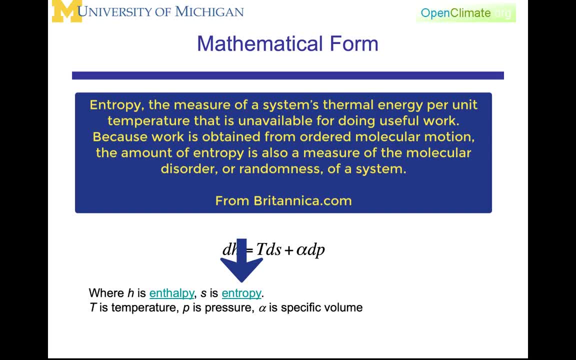 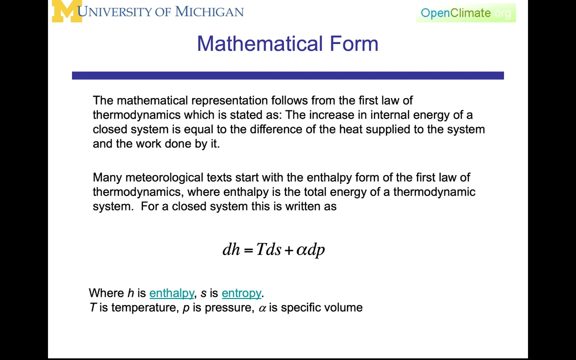 disorder. But there is a certain amount of internal energy within a substance that's not really available for work And hence the entropy appears as that sort of that base, that foundation, The change in entropy can be available for work. So again we're back to this idea of 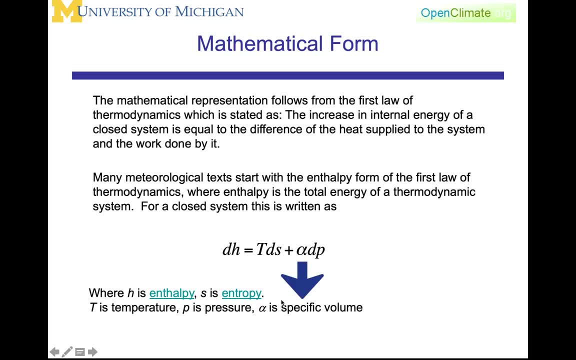 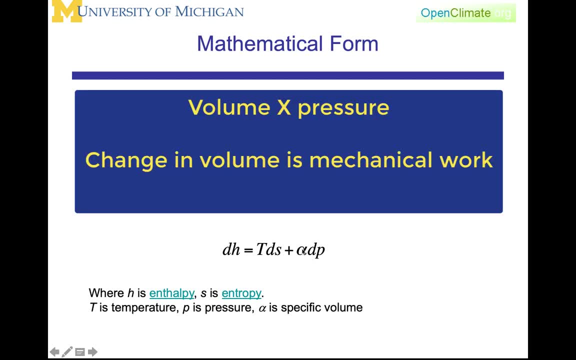 change. And then alpha is the specific volume, P is pressure And alpha dp is some sort of measure of volume times pressure which, if you can think of the volume as a measure of distance moved, you're talking about the relationship of mechanical energy.